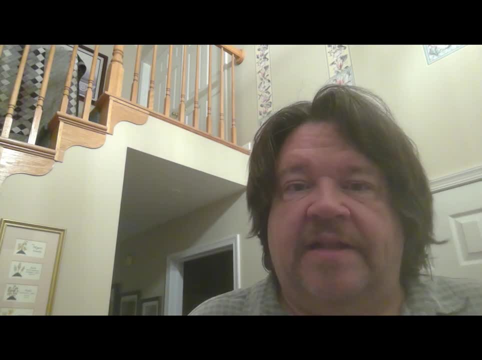 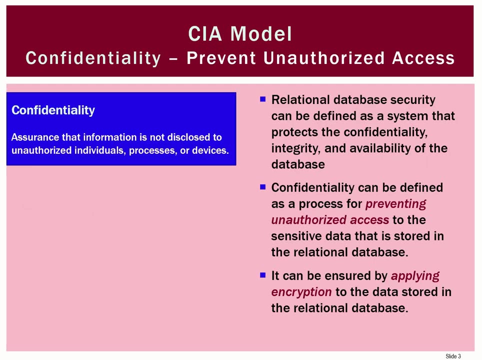 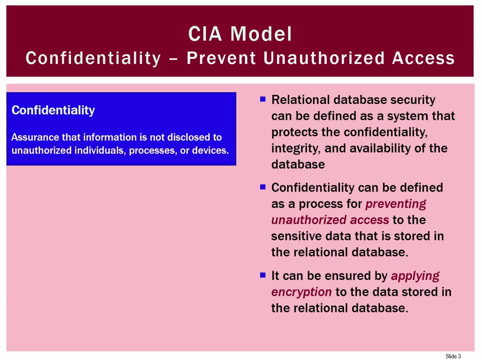 who is unauthorized, whether that be an individual, a process or a device. There are many ways to ensure confidentiality. You can use ACLs or permissions on tables to only expose the data to authorized users. You can use ACLs or permissions on tables to only expose the data to authorized users. 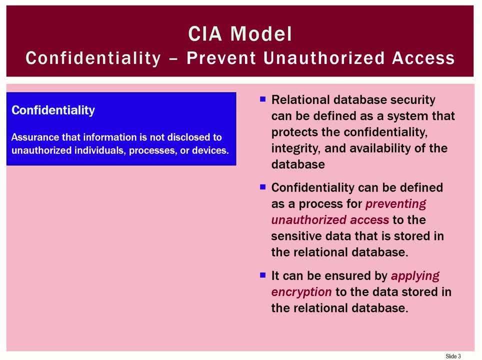 You can use ACLs or permissions on tables to only expose the data to authorized users. You can use views to hide certain columns that might be more confidential, Or you can apply encryption to the data that's stored in the database. These and other techniques will help guarantee that your data 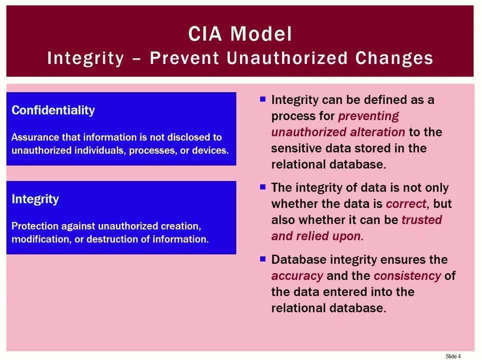 remains confidential. If confidentiality is protecting our data from being viewed by the wrong people, well then integrity is protecting our data from being modified by the wrong people. So integrity is the aspect where you can control your data. by an example, integrity provides controls on updating data, inserting data or deleting data. we 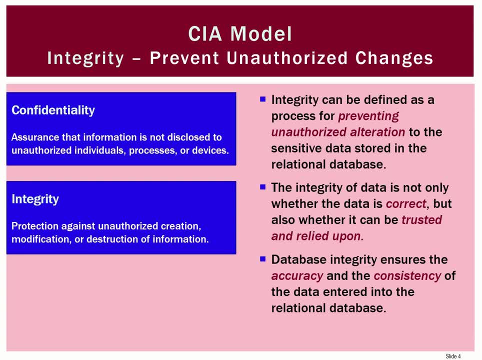 only want the right people, who have a custodial relationship to the data, to be performing such updates, inserts and deletes. typically, the number of users who can update, insert and delete is much smaller than the number of users who can select, so database integrity ensures the accuracy and the consistency of data. 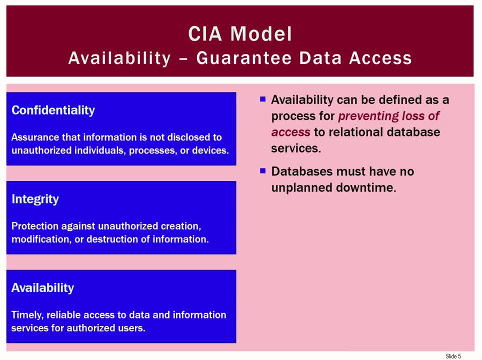 entered into your relational database. finally, we come to availability, and availability we define as timely, reliable access to data and information services for the authorized users. now you might be saying to yourself: why is availability so important? if the data is not available, like guess. it's the most secure of all. but the reason availability comes into play. 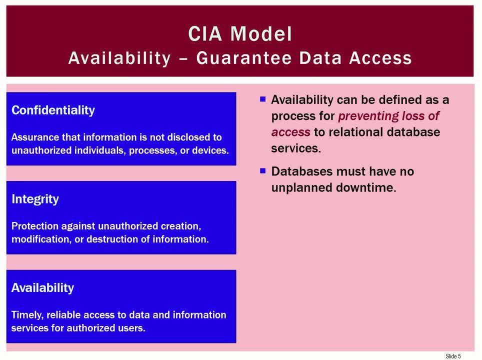 is that a lot of our data is needed in order to preserve the security of other systems. whether we're trying to preserve patient information by having a patient database where we can tell if a patient took a drug or a placebo, there's a lot more to security, beyond just the information itself. it's how the 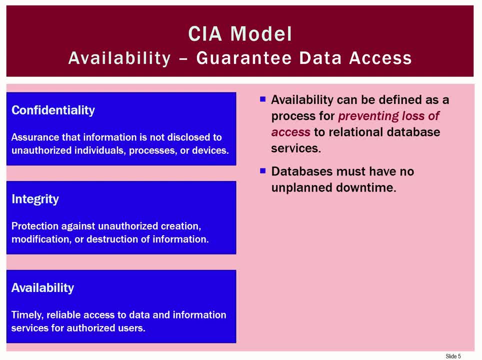 information is used, and if key information is not available to decision makers, they might make the wrong decision. so the availability of data most certainly is part of the CIA model, and we want to prevent loss of access to the relational database so that users can use the data as they see fit and when they see fit. that's. 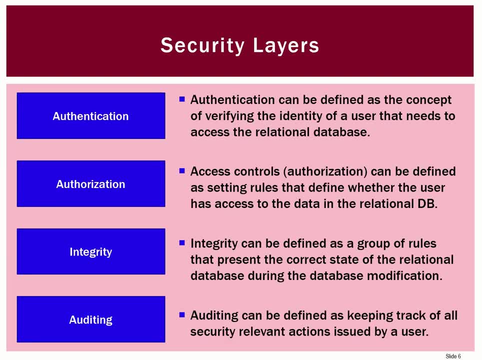 important consideration. as you will learn in cyber security classes, there are four security layers and, yes, integrity is repeated as one of those layers. let's discuss what these layers are. we start off with authentication. authentication means that we know who you are. we can verify your identity. this can be done with biometrics, can be done with strong passwords. 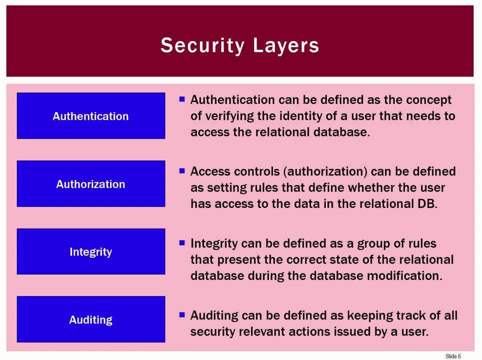 but we want to make sure that, when you are working with a relational database, that we know exactly who you are and no one is spoofing your identity. next, there is authorization, and this is important. we talked about acls before- access control lists- and these lists can be defined to determine whether a user has access to the data, either at the table level- 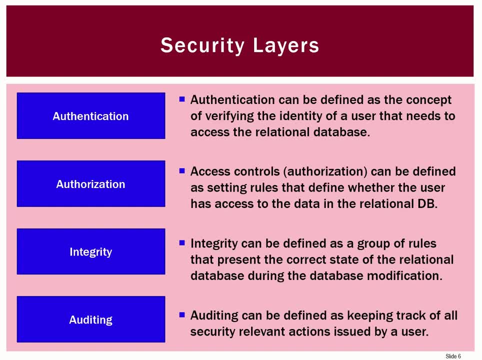 or at the uh column level. finally, there is two more layers. there's integrity, and integrity is a group of�만 rules that can protect the correct state of the database during its modifications. These rules can be enforced via triggers that can do some additional business logic checks. 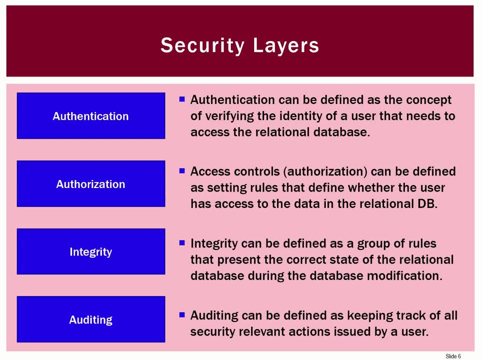 before data is changed. They can be enforced by using enums to limit the values that can be into a field. They can also be used simply by having good primary foreign key relationships and using the cascade on update and cascade on delete to ensure that when you do a data operation. 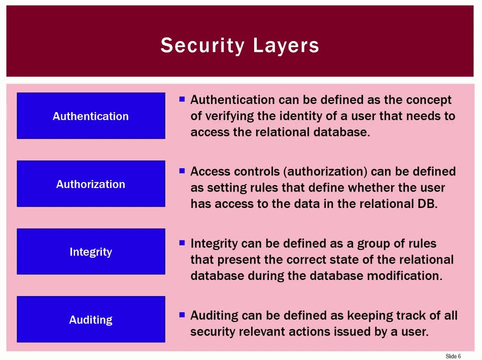 the database remains integral. And then, lastly, there's auditing. Auditing is really important. You want to keep track of all the actions done by a user. Auditing is often used to find suspicious behavior, unusual patterns of data access, And so, if the first three layers fail you. 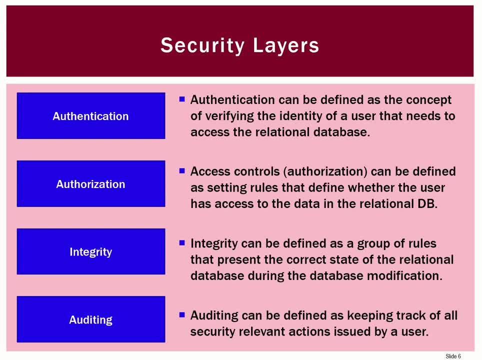 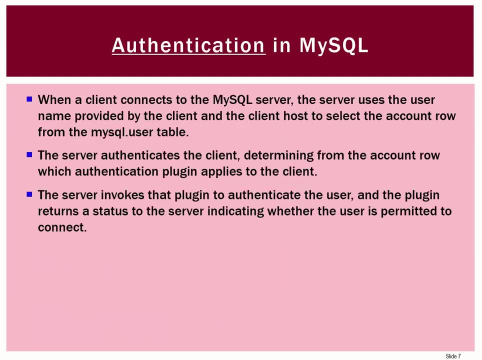 Auditing can help find suspicious behavior and help the DBAs and the IT people shut it down. So let's see how MySQL can offer some protections, especially for authentication and authorization. When it comes to authenticating, a user has to log in with a name provided and select. 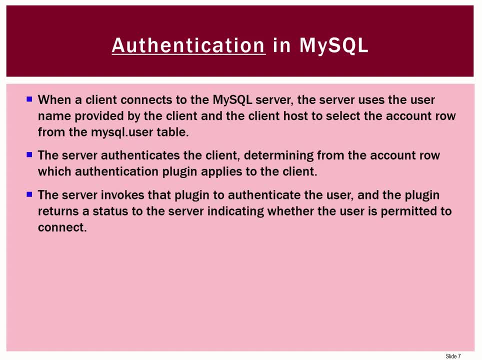 the client host. All the information about users is maintained in a special table, So you can see that the user has to log in with a name provided and select the client host. This is called the MySQLuser table. The server will then authenticate the client, determining from the account row which authentication. 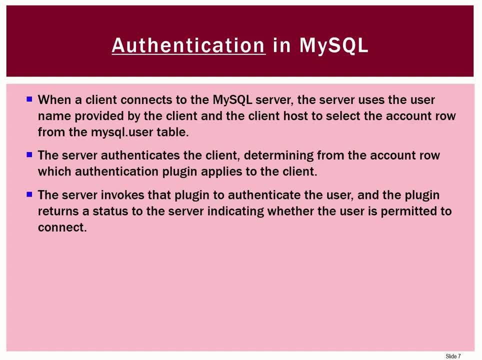 plug-in applies to the client And there are many different settings you can do in MySQL to make authentication more difficult. But at the end the server is going to invoke that plug-in, authenticate the user and then return a status indicating whether the user is permitted to connect. 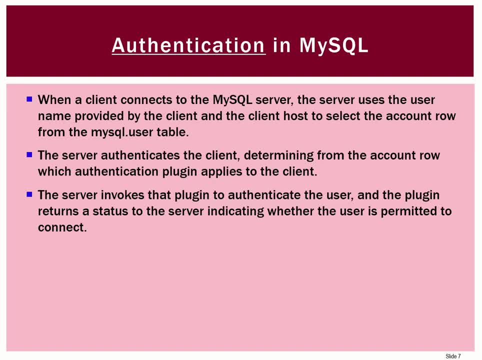 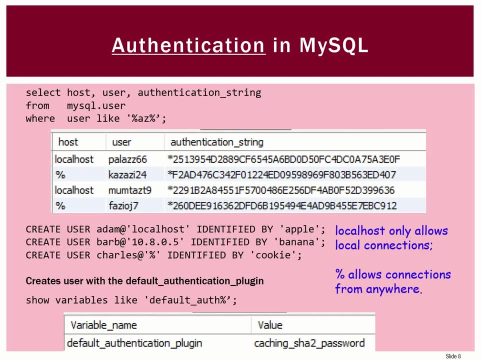 So that's a nice feature. this is your first layer of protection in MySQL, so let's look at some specifics about how authentication is managed behind the scenes in MySQL. and we have a query here that goes against that MySQL user table and it's bringing back the 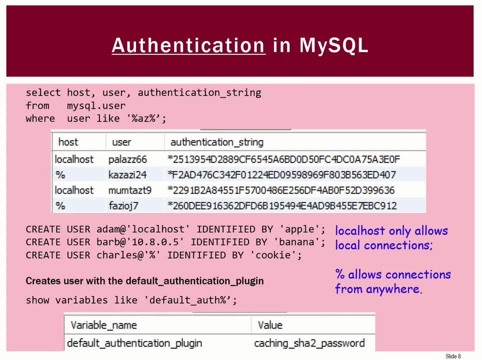 host, the user- and the authentication string, the user. column 2 is what you're familiar with. this is the username that you use to access MySQL. the local host in front of the user actually determines from where you can connect. we'll talk more about that in a second. and then there's the authentication string, the. 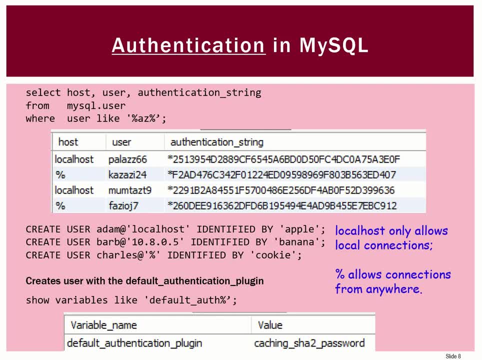 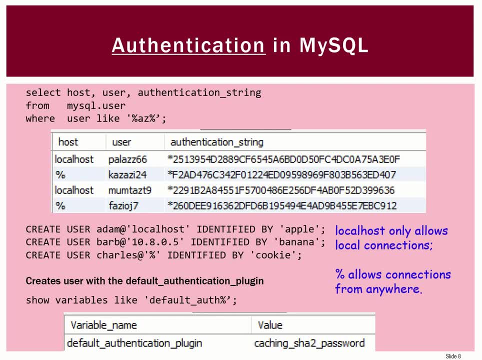 hash value And this is the way that you can protect passwords. So if Palaz66 calls up and says I forgot my password, can you tell me what it is? We, as database administrators, would be unable to do that because this is a one-way hash. We would just have to say: 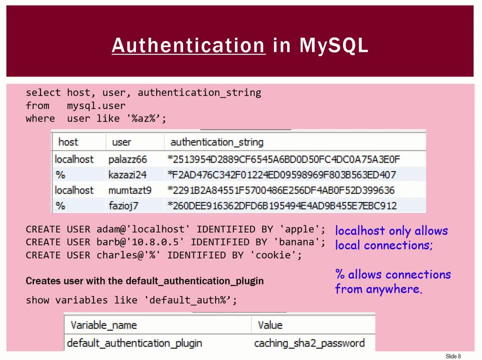 sorry, Palaz66, but we can reset your password and we can do that using the alter user commands. Okay, let's move down and look at our three create user statements. So we're going to create user Adam And what we're doing is we're saying at, and after the at are the locations from which 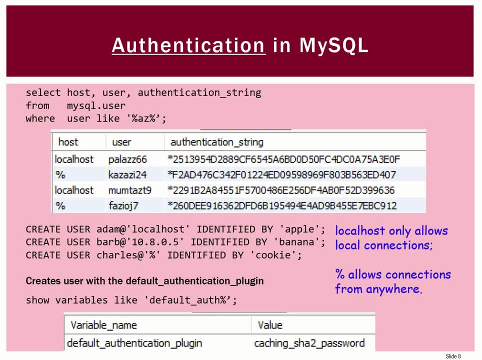 Adam can connect. So we created Adam at local host identified by Apple, probably not the best password, but just here for illustration. So what this means is that Adam can only connect from the machine itself. So we're going to create Adam at local host identified by Apple, probably not the 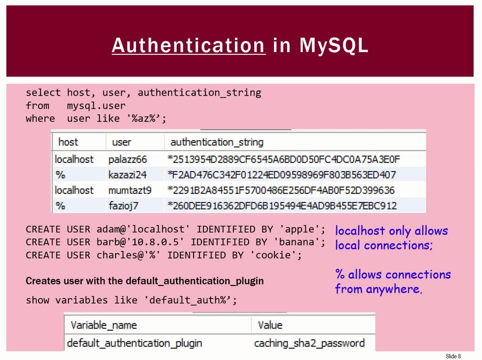 best password, but just here for illustration. So we're going to create Adam at local host identified by Apple. he can't connect to it through web services or anything else. He must be logged on to the database server in order to connect. By the way, if you don't specify the at and the location, 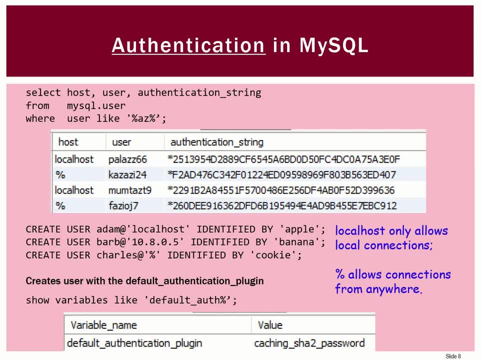 after it, you will automatically default to local host. Now let's look at Barb. Barb is very interesting. When we created Barb, we identified a very specific IP address, So Barb can only connect to the database server in order to connect. So we're going to create a very specific IP. 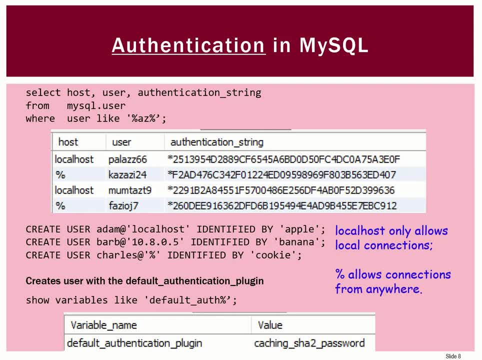 connect to the database from 10.8.0.5.. She can't connect from any other IP address. This is really locking Barb down and perhaps is the most secure but the hardest to predict, because who knows where Barb will need to log in from. 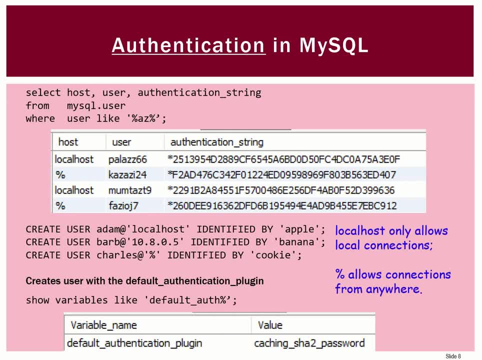 And then we've created Charles. Charles is created with the wildcard, the percent sign as the host, and the percent sign allows connections from anywhere. So this is how you would create users, And if you wanted to change a user's password, you would just substitute the word create with the word alter and the syntax would be: 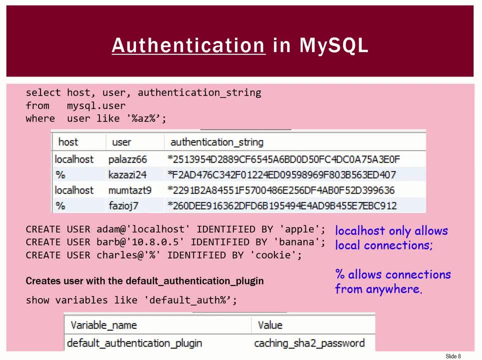 the same Now. we talked earlier about the different ways you could authenticate, And one of those is a user variable for MySQL, And so we're looking at the name default authentication plugin, and you have many different options for this: to improve your security or to select the hashing algorithm that you want to use. In this case, we're 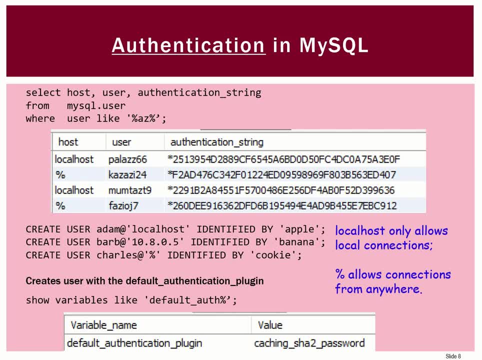 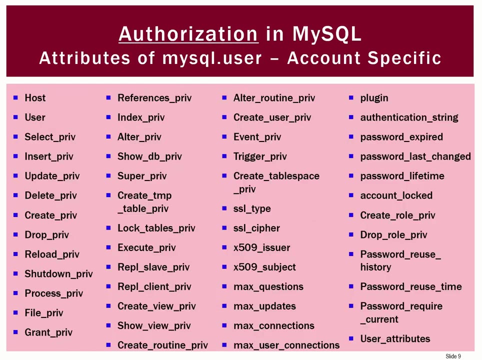 using an SHA2 algorithm to hash the password, but there are other values you can choose. So this is some examples of how we can, as DBAs, set up our users with the correct passwords, the correct locations to connect from and the correct approach to hashing their passwords. 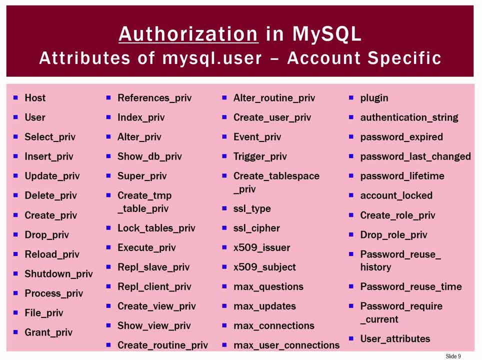 So let's move on to authorization now And remember, authorization says that a user has the right roles or the right privileges, And we're not going to go through all of these different options, but look at these attributes of a user. You can determine whether a user can only do select statements or whether they can do. 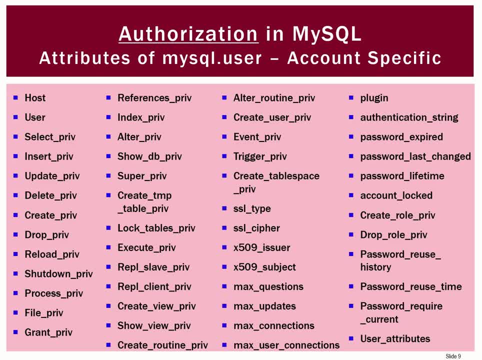 inserts or updates Or deletes, creating tables, dropping tables, shutting down the database, altering privileges, locking tables. There's many different controls you can place on a user so that they have the right permissions. Don't just give every single user select, insert, update and delete privileges. 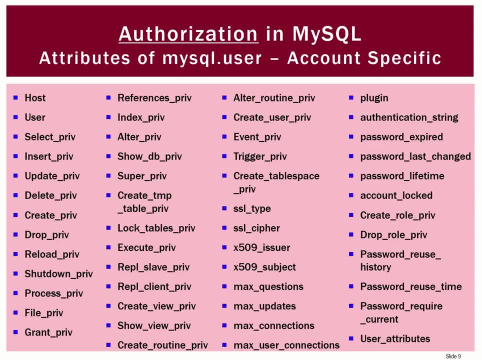 Maybe you only want to give them select and insert, Maybe they can't delete data. So think about your users. think about what's the most secure way to have them be authorized in terms of their roles. You can look these up, you can see what these do and then develop security policies. so 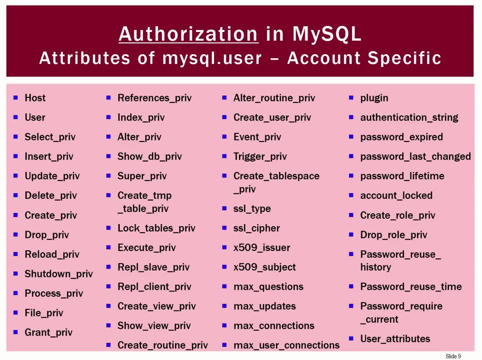 that users can do only exactly what you want them to do, And these attributes apply to the entire user. So if you said a user did not have deletes, If you said a user did not have delete privileges, then a user could not delete from any table. 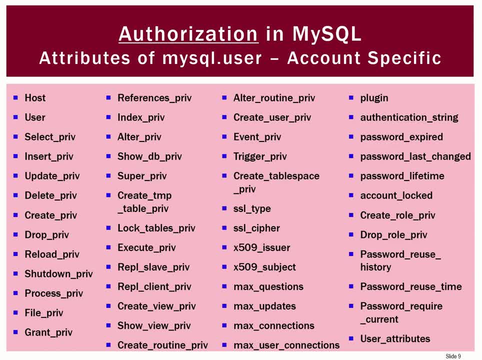 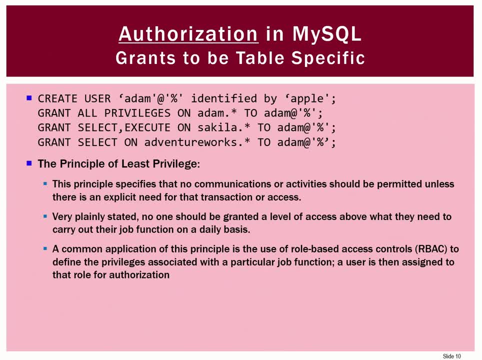 in the database. If you said the user did not have drop privileges, then a user could not drop any tables. So if the previous slide referred to authorization of a user across all tables, you can also be more granular with authorization and you can have authorization that is table specific. 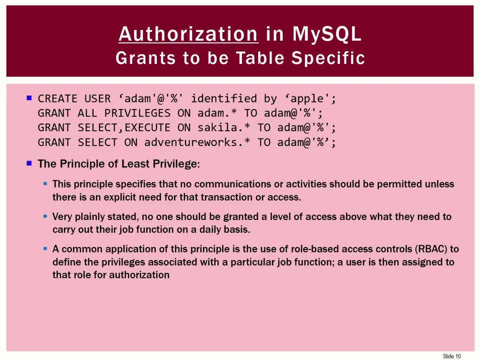 So here is Adam, who we created before, And we can grant all privileges on Adam to his own schema. That's what the first grant is doing. We can also look at other schemas. Here's the Sakela database. Maybe for the Sakela database we want Adam to be able to select and run some stored procedures. 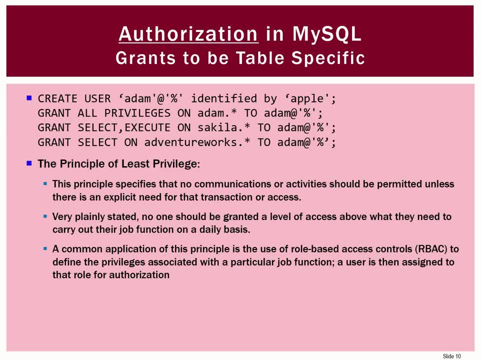 but that's it. So we can grant him, select and execute on Sakela. And here is Adam As he applies. He applies to the AdventureWorks database and maybe for the AdventureWorks database. all we want Adam to do is select. 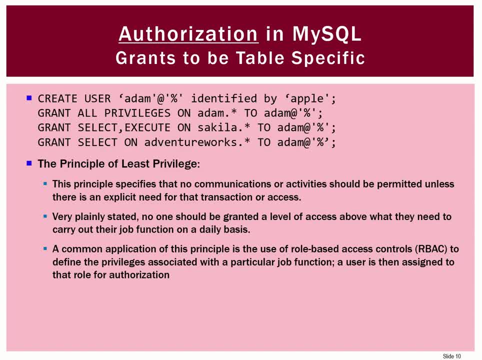 And so we're going to conclude with this prevailing concept, really very important for security. It's called the principle of least privilege And it's kind of a need to know basis or really a need to do basis. So the principle specifies that no activity should be permitted unless there is a need. 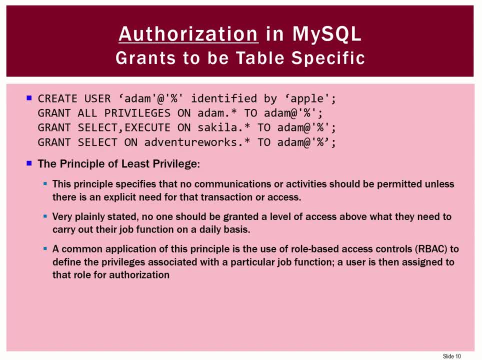 is an explicit need for that transaction, In other words, access. you are guilty unless proven innocent. It's better to make an error, to be more conservative and more strict than it is to be too lenient with security. So, in other words, nobody should be granted a level of access above what they need to. 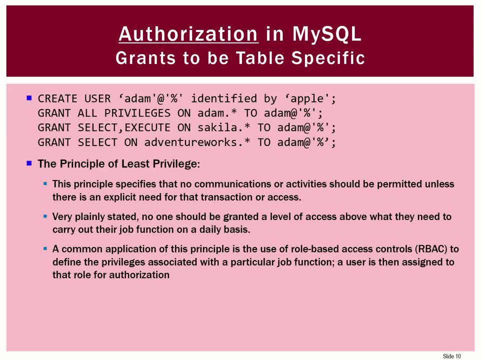 carry out their job function on a daily basis And with MySQL. Well, It's called role based access controls, And what we can do is we can use this is called our back. We can use our back to collect lots of privileges and group them into a role. 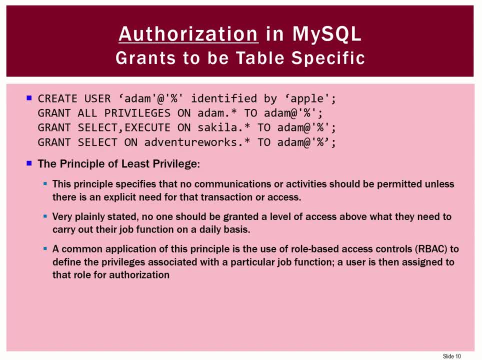 So, for example, anyone who's in the HR department might have these privileges on a set of tables. Anyone in the IT department might have a different set of privileges, And you can granularize this to the department level and or to the role level.